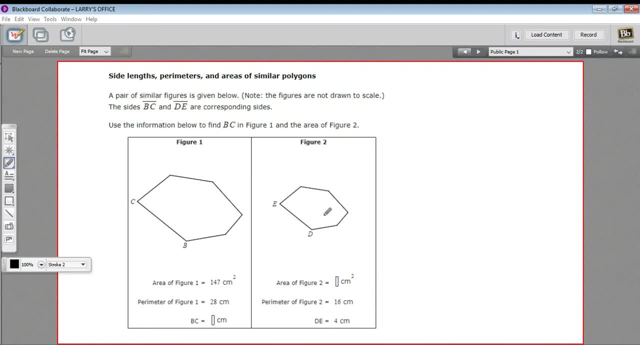 In this problem we are comparing side lengths, perimeters and areas of similar polygons. So we've got two polygons and they're proportional to each other. So this is just a smaller version of this one. So by however much this side is smaller than this side, then all the sides. 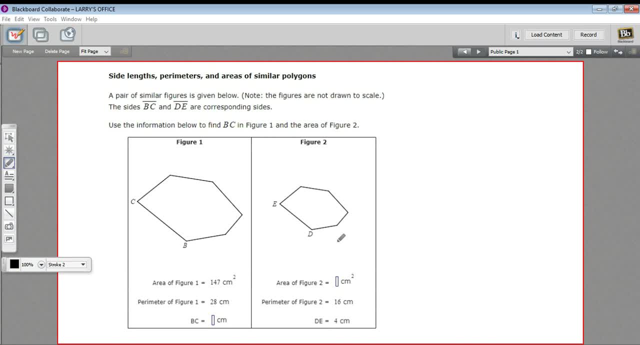 are that same degree smaller. So we've been given the perimeter for both of these, but only a side for one and only- sorry- an area for one and only a side for one, And we want to fill in the blanks for the rest of this stuff. We've really got two separate kinds of measurements here. We've got 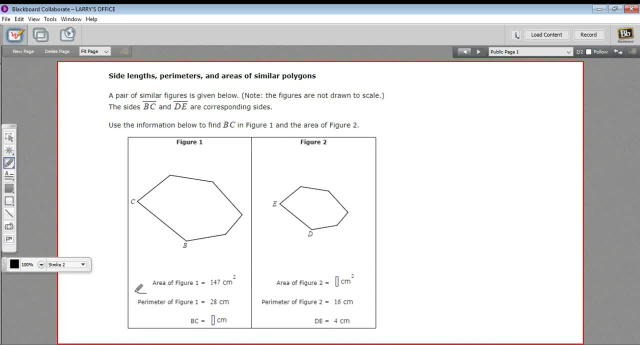 measurements of length and a measurement of area. So these two, the side length and the perimeter, are measurements of length. This one, the area, that's a little bit different. It's going to be treated differently. So let's just start with these measurements of length. First of all, we've got 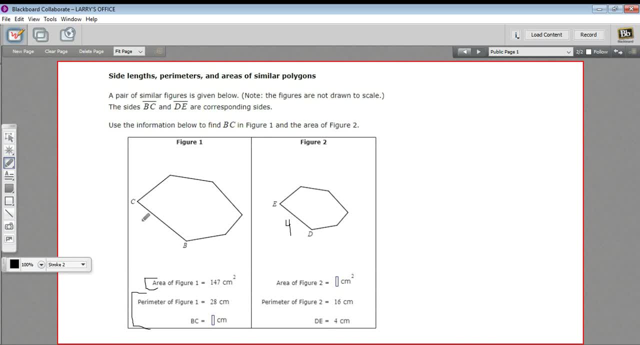 side length and the perimeter. So we've got side length and the perimeter. So we've got side length. side d, e is four, but we don't know what side c, b is And we're trying to get that. But we are given the perimeter of this larger one. This is 28.. So all the way around is 28. And this one. 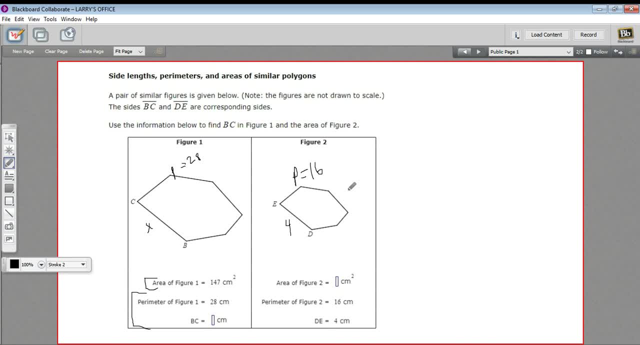 the perimeter is 16.. We can use those two measurements to create a ratio to show how these two similar polygons are related and use that to set up proportions to solve for the side. So let's just put the big polygon on top, So that's a perimeter of 28. And the smaller 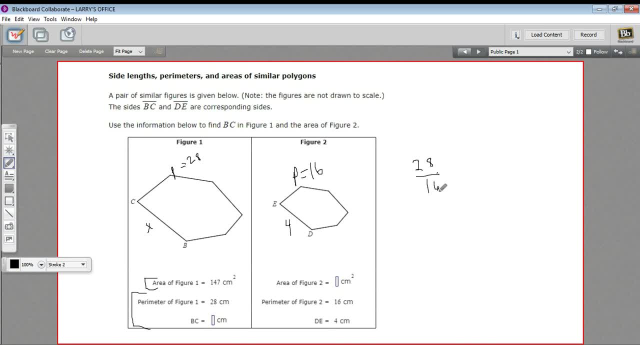 polygon on the bottom perimeter of 16.. And then let's just simplify this. Let's see: both of those are divisible by four, So seven fourths. So this polygon is seven fourths. all the sides are seven fourths bigger than this one. So if we want to solve for this side here of the bigger polygon, 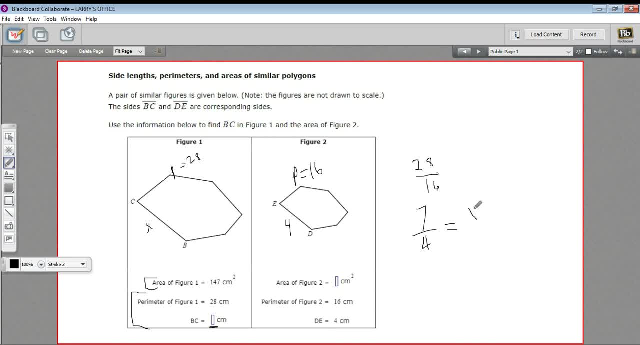 we'd set up a proportion with seven fourths on one side and x over four on the other side. In a proportion you have to have things in the same order. I've got big polygon, little polygon. big polygon, little polygon. 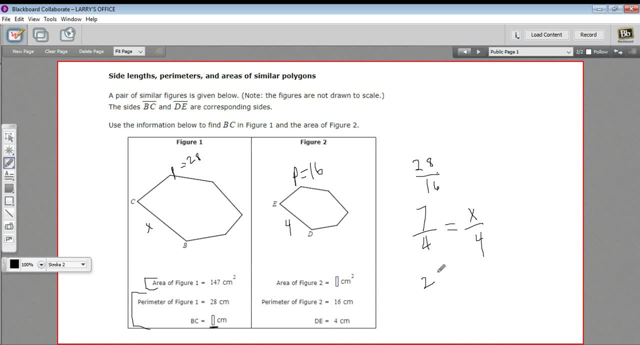 If we solve this seven times four is 28.. And then four times x is 4x And we divide by four- you may have done this in your head already- and you get x equals seven. So this side is seven. We can fill that in down here. So we've solved that, The other piece we need to fill in. 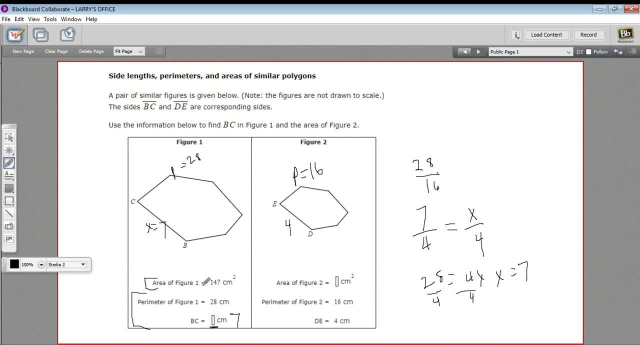 here is the area of the smaller polygon. We've got the area of the larger polygon. I said that area was a different kind of measure. We can't just use this seven fourths to solve the area in the same way. The reason is that area is units squared, So what we need to do is take this guy right here. and square it, And that's what we're going to do. So we're going to take this guy right here and square it, And that's what we're going to do. And that's what we're going to do, And that's what. 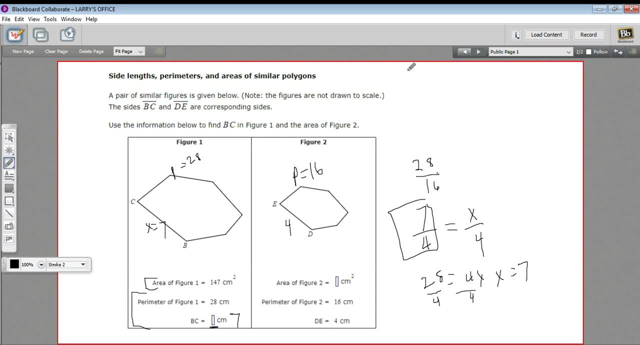 we're going to use to set up our proportion. So 7 fourths squared is going to equal. then we'll set up the same ratio: a large polygon on top, So 147 over a small polygon. that's the one we're looking for. So let's do some simplification here. If I square 7 fourths, 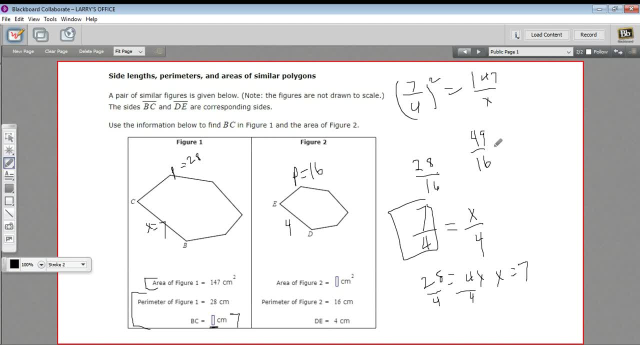 I get 49 over 16.. And here I've got 147 over x and I can cross multiply. So 49 times x equals and 16 times 147, I'm going to need to pull up my calculator for that times 147. 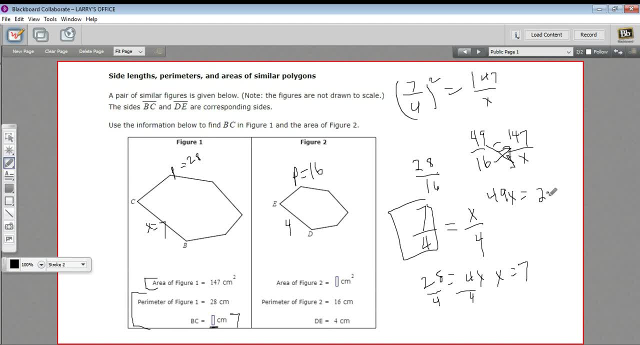 And I get 2352.. And then to solve for x, I'm going to need to multiply by x. For x, we need to divide both sides by 49. So we'll divide that by 49, and I'm getting x equals 48. And this is in centimeters. 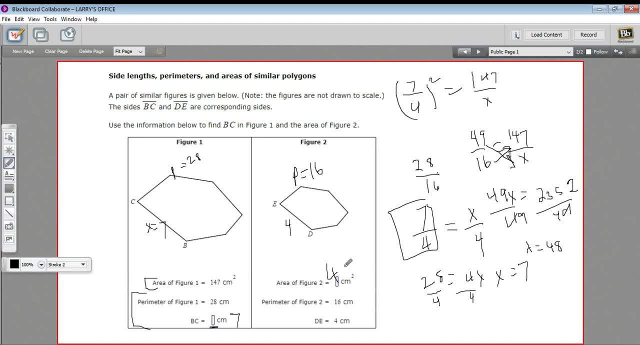 so that's centimeters squared and we can put our 48 in right here. So perimeter side lengths- both just measures of length. Just set up your proportion like you're used to With area. you need to just square this ratio. 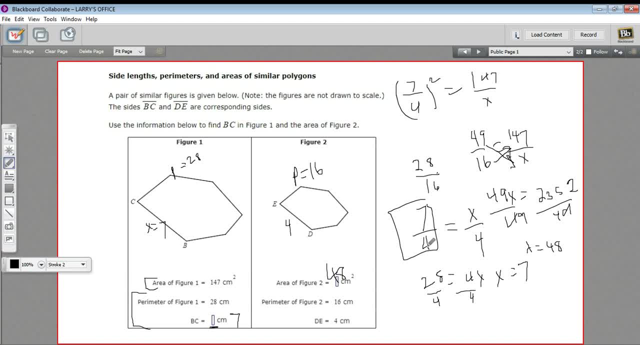 So that's a little bit of work with finding side lengths, perimeters and areas in similar polygons.